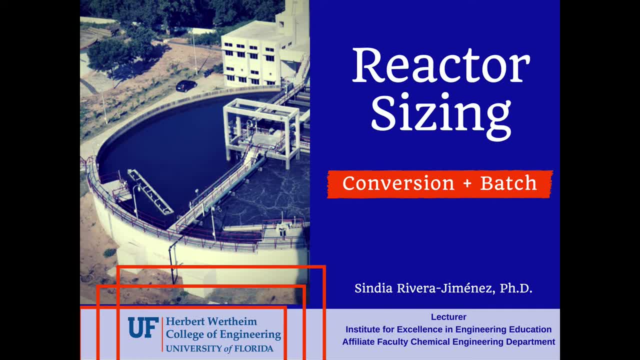 are very, very common in this industry. This is a sequenced batch reactor system, so while one reactor- the one on the right- is working, then the other one is shut down. Probably you can just unload it and then the other one is being on working operation. 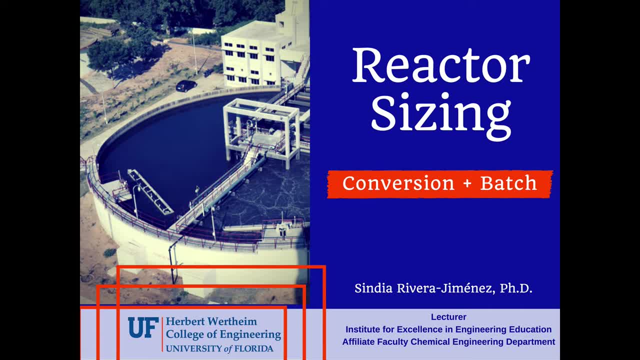 at the same time. So this is a way of maximizing the space available in the facility. This particular topic that we're going to be talking about will have some main goals. The first one is that we're going to go all over again the balance equation. 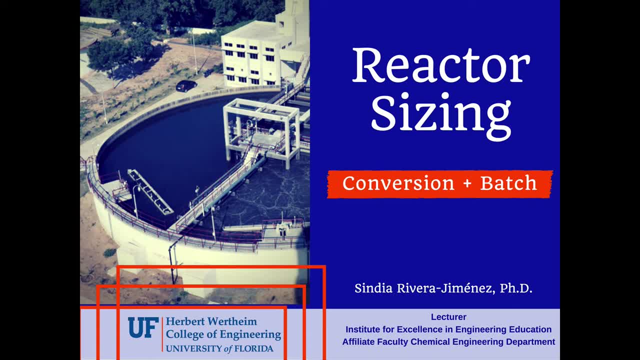 In terms. now on conversion, this time I'm going to be skipping some steps and we're going to go to the conclusion that the same analysis can be performed as we did before with mole balances. The other thing that we're going to do is that we are going to size the 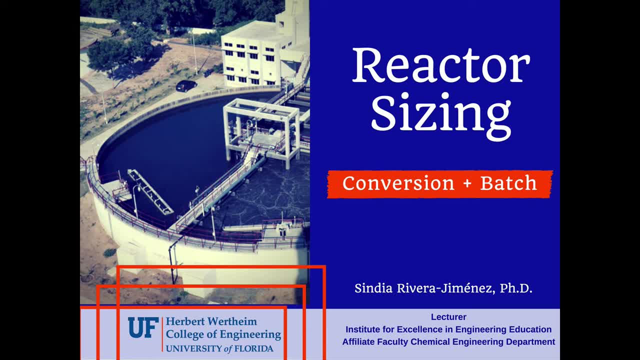 reactors given the rate of reaction of the limiting reactant or one of the reactants as a function of conversion. We're going to see examples comparing CSTRs and PFRs and we're going to be deciding the best arrangement for reactors in series to maximize conversion, and we're going to be 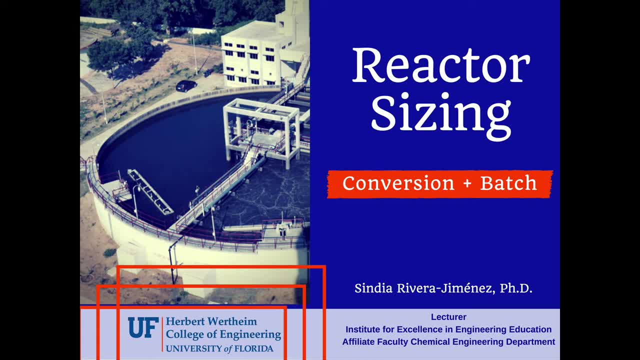 calculating the overall conversion of reactors volumes for reactors arranged in series. This is going to be a sequence of a couple of videos and the idea is that we mix them up. We mixed up different types of reactors. We tried to get various of them mixed up. We tried to get different types of reactors. I tried to get them mixed up. We mixed up different types of reactors. We tried to get. 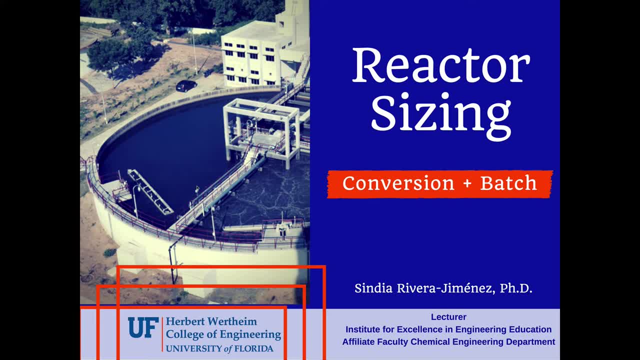 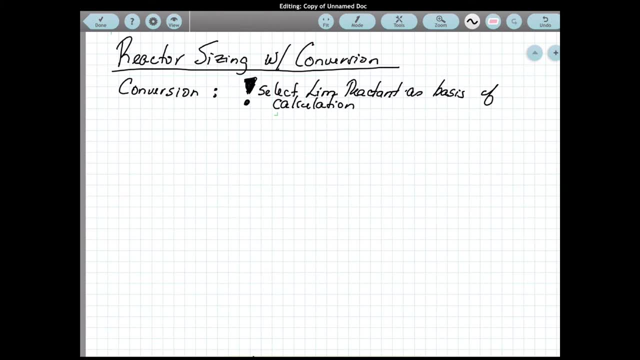 or maximize conversion. So this section of the class is gonna be really fun. So let's start with the definition of conversion. For conversion, we need to select reactant. typically, or most commonly, is the limiting reactant as the basis of calculation. Remember that once you have the conversion for 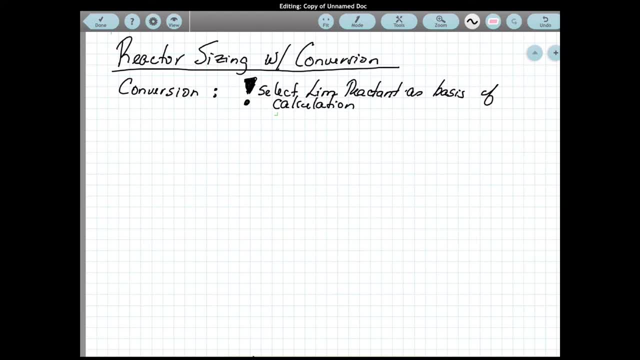 one reactant. you can use the stoichiometry pretty much to relate this conversion to other species in the chemical reaction. It is important that we choose the limiting reactant because technically is the reactant that will be completely consumed first, after the reactant has been mixed. therefore, 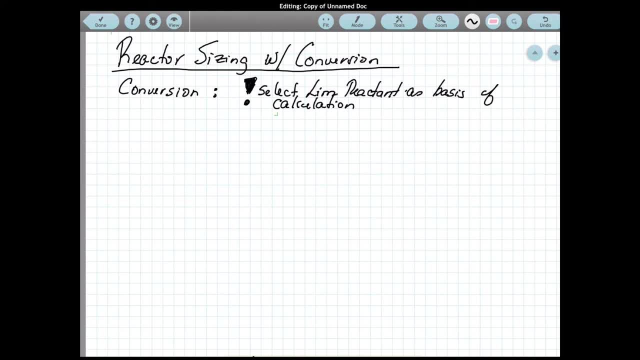 provides more information about the reaction. Okay, so let's start with a general reaction. This reaction, we're gonna select A as our limiting reactant and to have you know the chemical reaction defined as in terms of the chemical reactant, What? 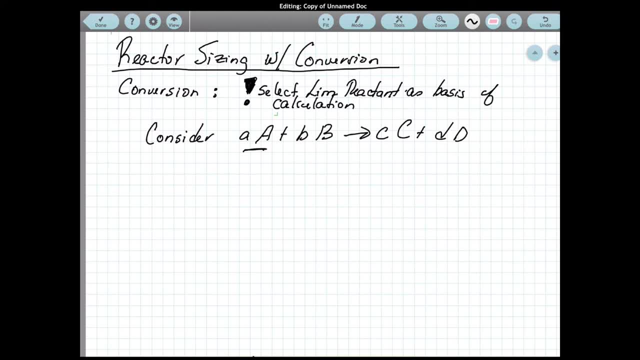 we're gonna do is that we're gonna normalize the chemical reaction for one mole of the chemical reactant, so we're gonna have a chemical equation that will have will look like this: okay, so that means that we can define conversion as capital. x equals to the moles of a. 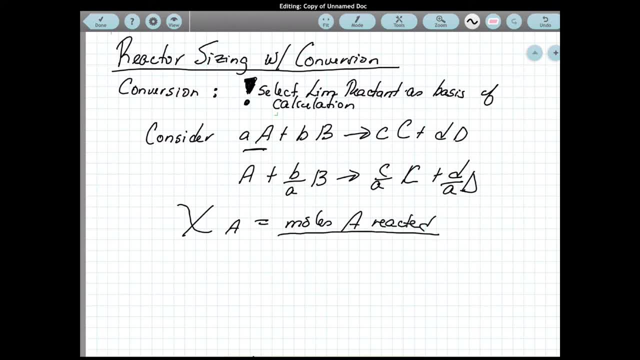 reacted over the moles of a fed into the system. okay, this is an important quantity because it tells us information about how far the reaction proceeds to product. we can actually see that. we can also collect the reactants into a just long variable river and when we track that we can see. something we have to see that it flows to a short river line, okay, and when it flows to a short river- saline, cualum dalli- ok, we can actually. we can protect or significantly monitor the ACEP PRODUCTION, okay, and you can actually let go of it. we can also follow up as we go along with this, you could. 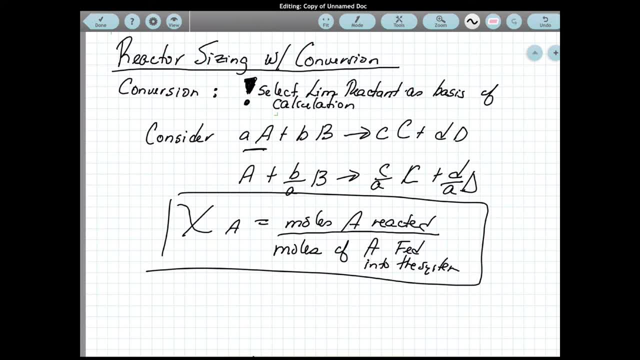 relate this to any other species in the chemical reaction. you can drop the subscript. you get to see it that I just dropped the substrate, because one of the assumptions when we develop this equation is that A is the limiting reactant. so once you know the limiting reactant, you can- you can just define AX. 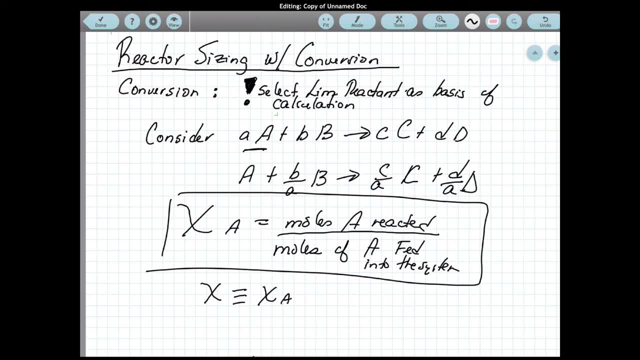 right instead of. instead of using XA, I will use those terms. you know it will depend right on the type of problem that I'm solving. there are important things to consider when we have the conversion definition. one is that for irreversible reactions, reactions where the equilibrium constant K right is. 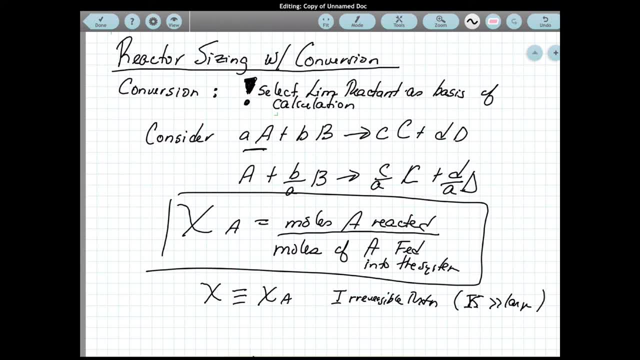 really, really large. the maximum conversion that we can have. X maximum equals to or is close to right- not always equal- is close to 1.0, 1.0. for, for a reversible reaction, X max conversion maximum equals to the X at equilibrium. okay, we're gonna. we're gonna see examples for both, but it's 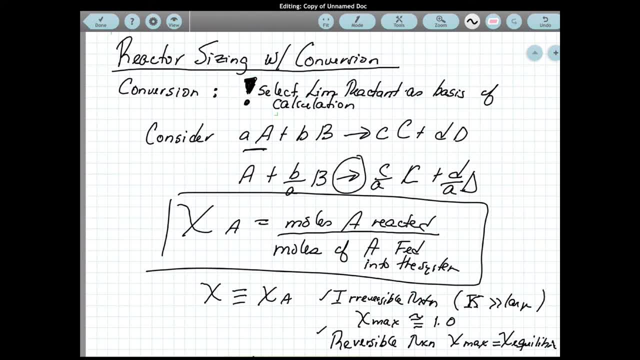 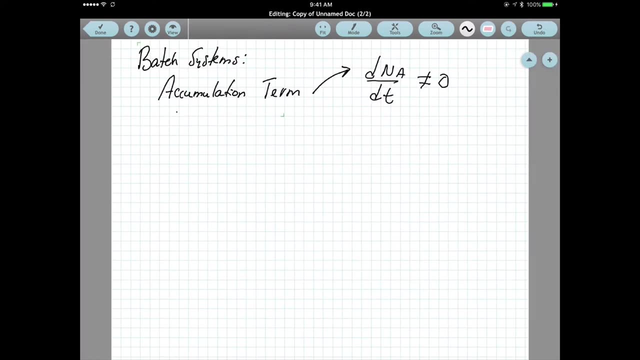 important that we look at the chemical reaction right and the identity of that chemical reaction to kind of understand or guide us on what is the maximum amount of conversion we can have for that particular reaction. so for batch systems we can define or we can assume right that the accumulation terms 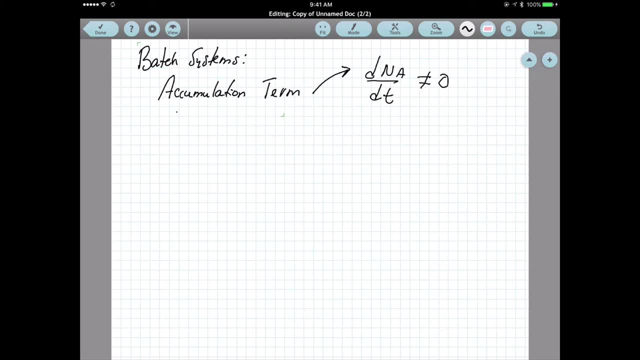 are different from zero for the mass balance. that means that for the mass balance this term is going to be important. so we need to take define what is NA and see if we can find an expression right on the number of mole in terms of conversion. so we know that NA right can be defined as the moles. 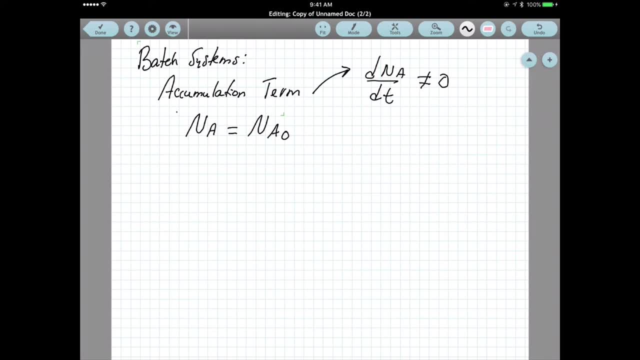 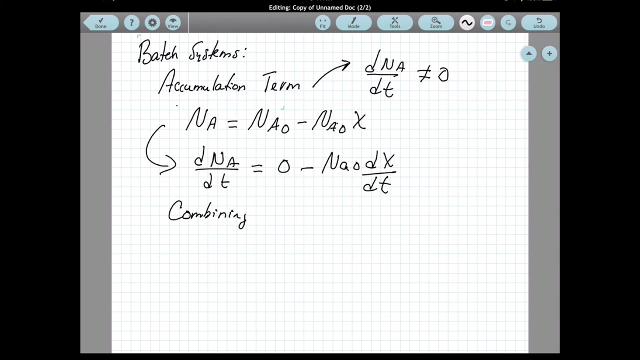 entering the initially in the reactor, not entering initially in the reactor in the reactor, minus whatever reacted of species A. okay, We can then take this term and try to get the derivative form right And we can see that with respect, time and combining. we have remember that the sign is because we 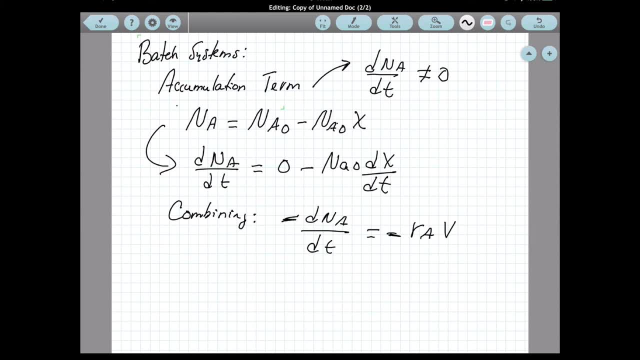 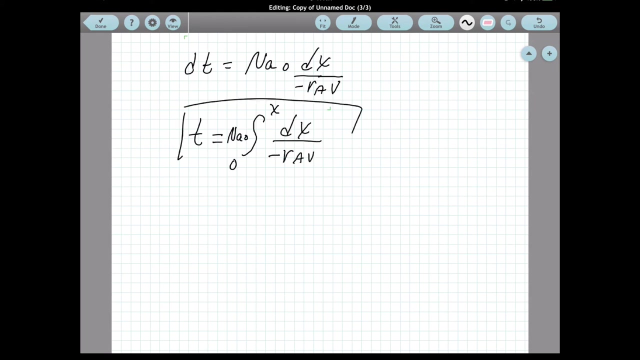 are. we know that it's our reactant that is not being accumulated, it is being produced, and we are arranging in direct line, Separating variables and alternating Verb. There we go. Good for that. What do we need? and integration provides the parameter for the batch reactor. okay, this will be. 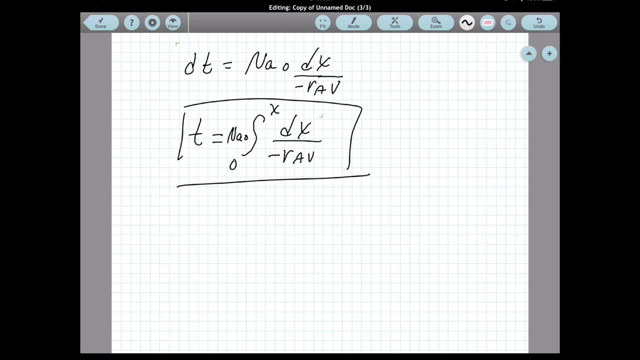 the time necessary to achieve a conversion of X in a batch reactor. notice that the longer the reactants are left in the reactor, the greater the conversion will be. we can also represent this, this equation, in a graphical form. right, if we grab any initial moles of a? 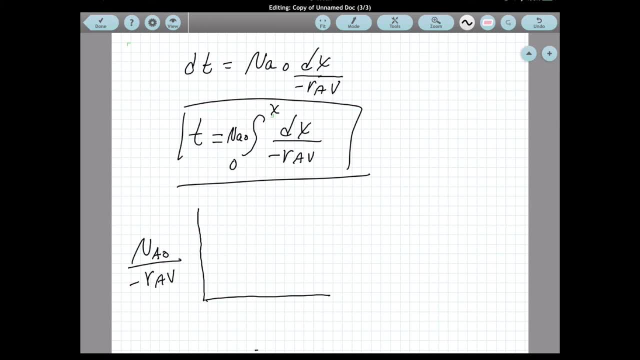 remember that this is also the initial concentration of a. we get a graph that looks something like this kind of: yeah, it looks something like that, and if I'm trying by, this is X, try to get at a specific conversion. oops, trying to get up to look at a specific conversion like this one, right? 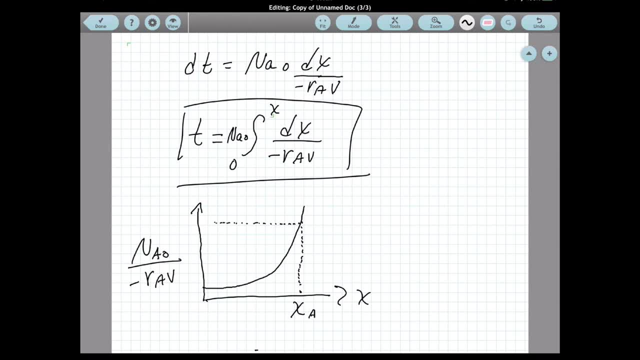 and then we look at the corresponding conversion, like this right, and then we look at the y-axis right, because this equation is in the form of an integral. we can see that the, the, the area right under, corresponds to T or the time. so if we have data collected for that particular reactor, we can actually 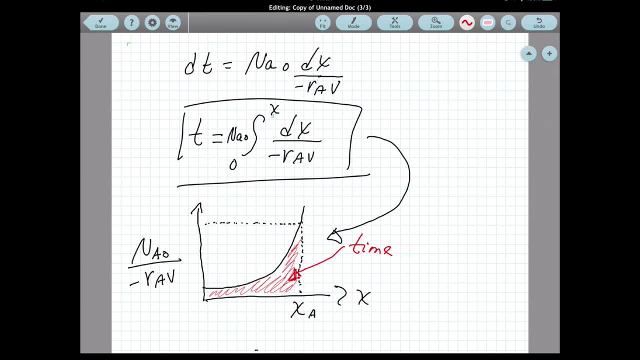 rearrange the parameters so they look like this type of graph and we can graphically calculate the time of the reactor.